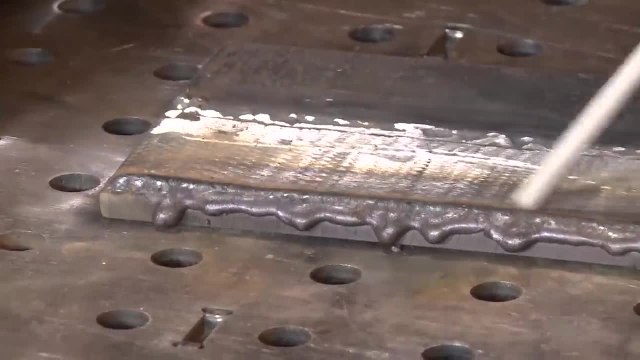 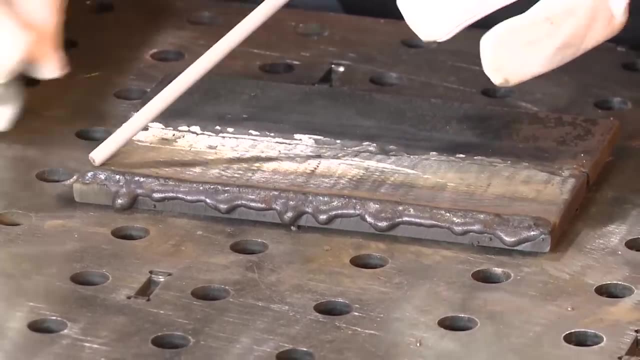 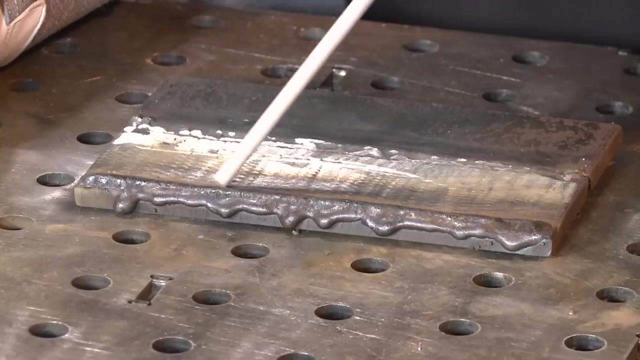 this weld about halfway up and I want to run a straight line. Same width, same height. If I change my travel speed and start going real slow, this bead is going to widen out. If I change my travel speed and race forward, the bead is going to narrow up a little bit. 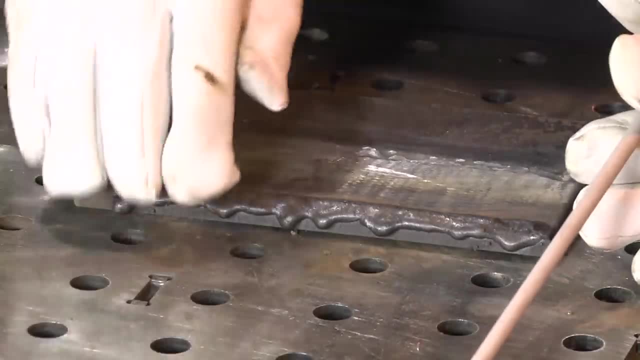 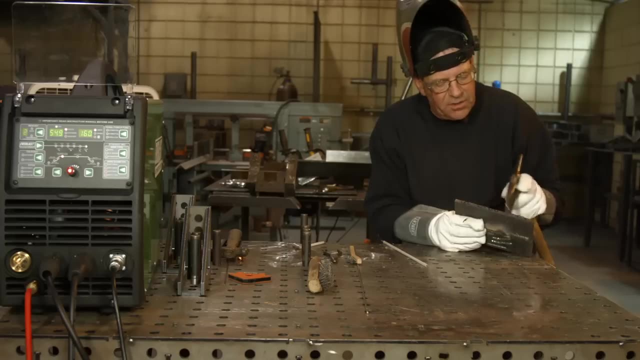 I'm not going to get the blend either. By the way, if you're looking at this on the camera and you're thinking, wow, that's rough, that looks stupid, it probably does, because it's got slag dripped over the edge. I'll clean that up after a while, Matter of fact. 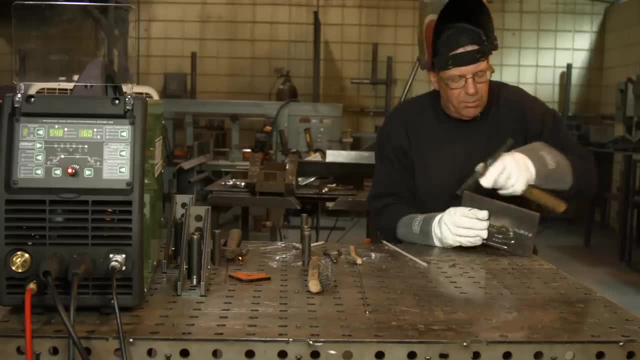 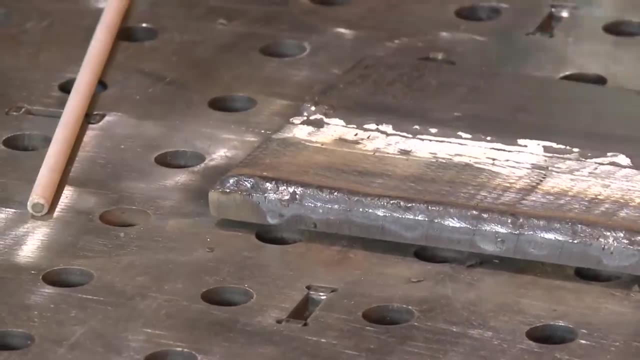 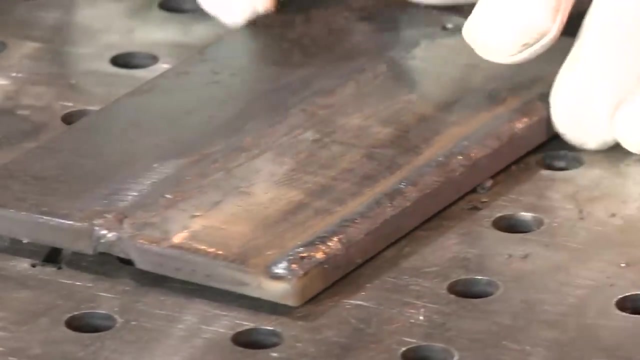 I can clean that up while I'm talking to you. Boom, I'm done. Edge of that weld is barely hanging over the edge of the plate there. Bad habits, bad habits to get into is to weld habits, bad habits to get into is to weld toward yourself, I think. anyway, you know. 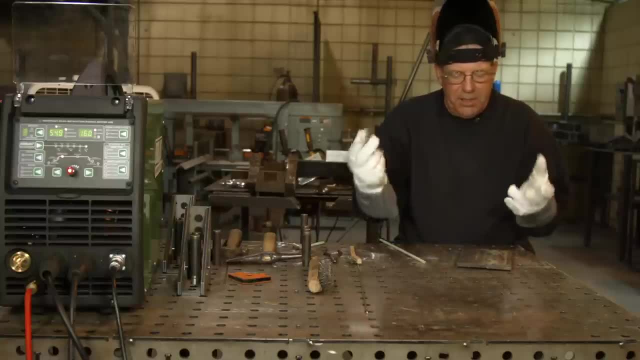 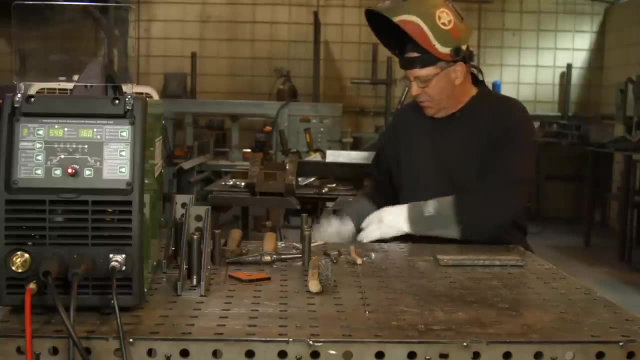 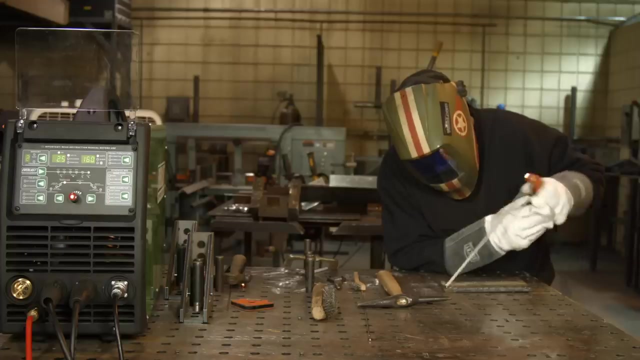 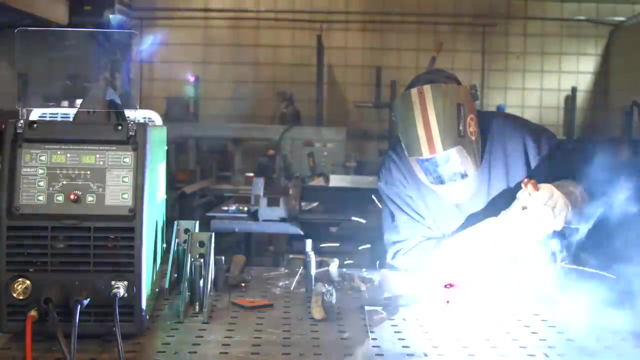 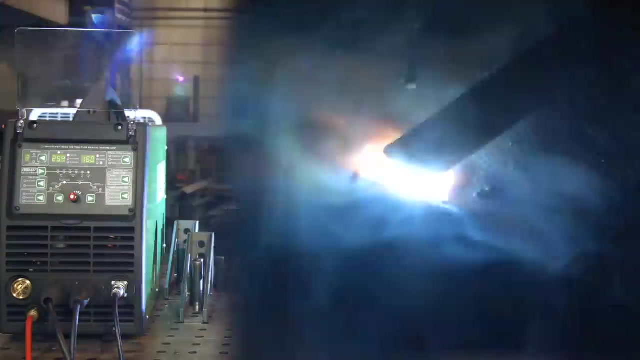 later on we will learn how to manipulate in all positions and everything, but right now, let's just let's concentrate on doing this, and hopefully we'll see some slag peel out of it too. come on, darling light up here, don't be that way. here we go. I need to explain what I'm seeing, what I'm feeling here. I have this. 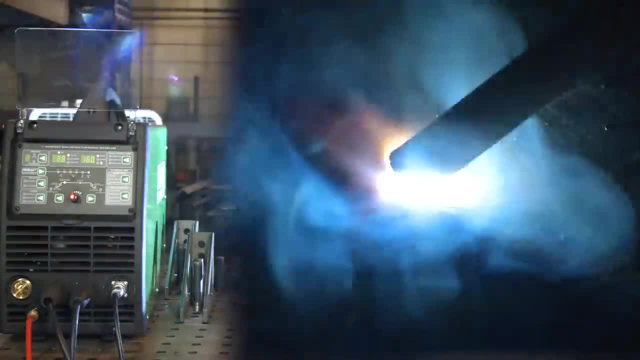 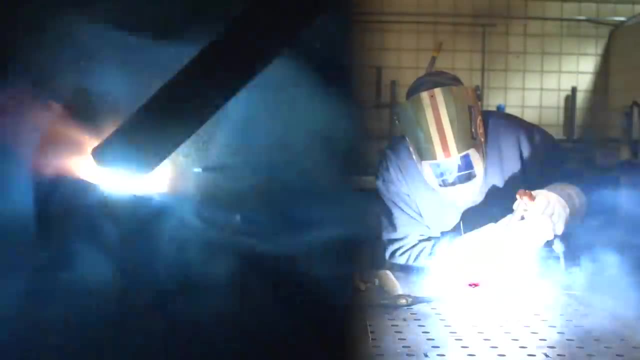 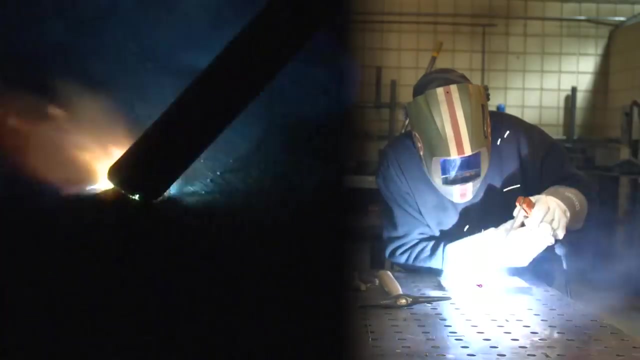 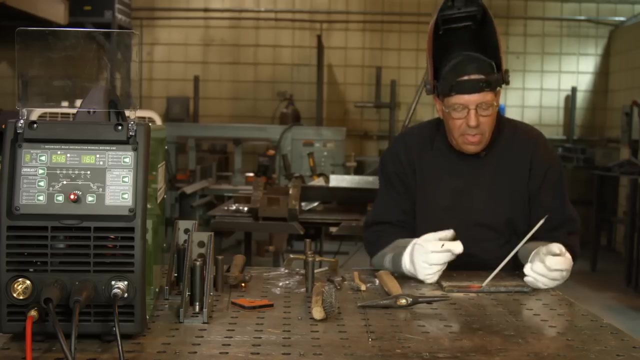 rod leaned back probably about 40 degrees or so. I also have it pointed toward me about 10 degrees, just so I can get that slag. running behind me the whole weld pool, and I'm barely touching the plate. I can feel the plate. whoo, there we go. welcome to stick welding. I see what? 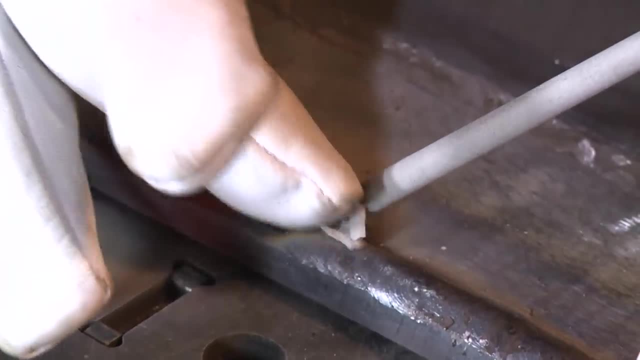 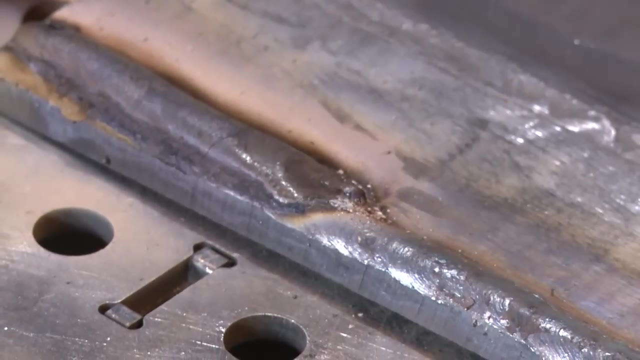 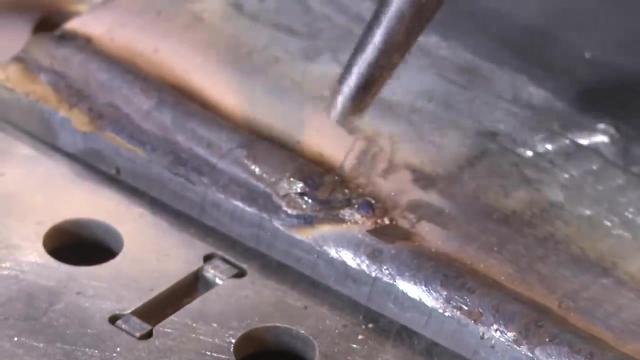 happened here. I've got a big old crack in my slag here. it just kind of fell off so I've got an electrode that, hmm, not good, not good, not good got an electrode. you need to check the flux on them. I found some here lately that I found a 6010 the other day, a 6010 the other day that had about a. 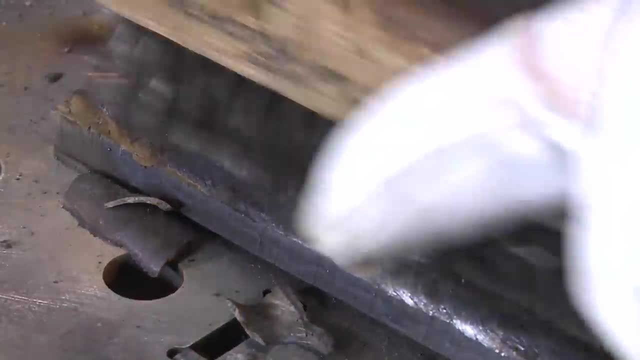 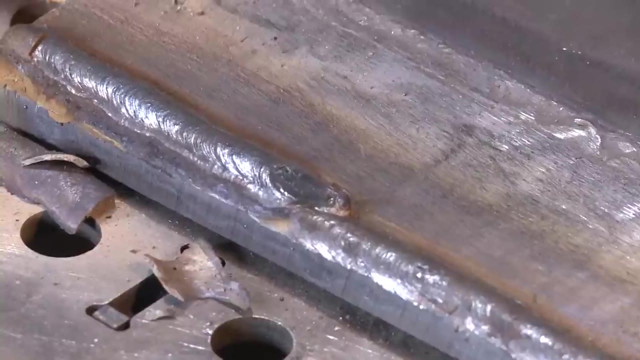 third of the way up from the start of the rod. I'm gonna leave that little dingus on there and see if I can weld over the top of it. when I restrike this rod, I want to restrike it out here in the direction that I'm going. I want to. 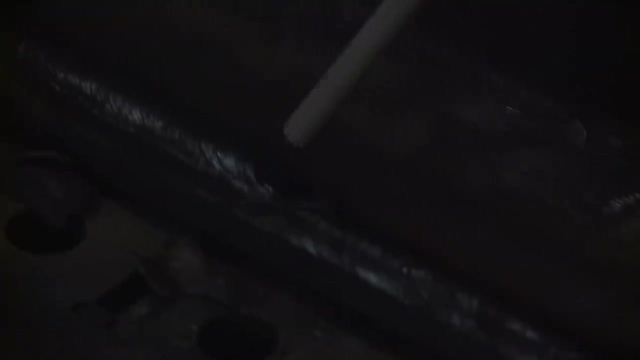 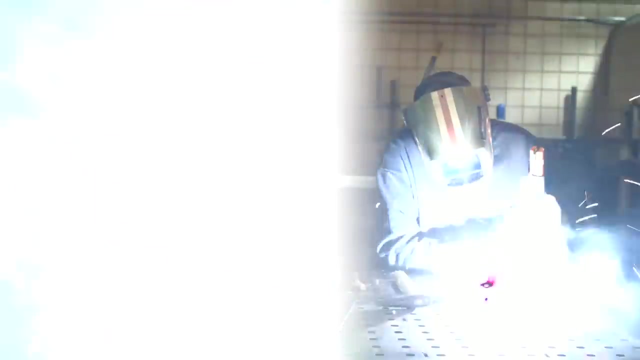 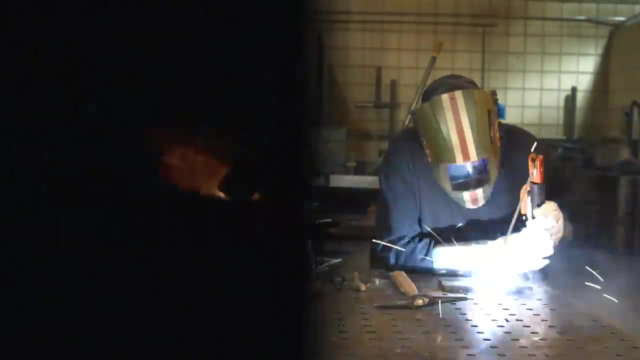 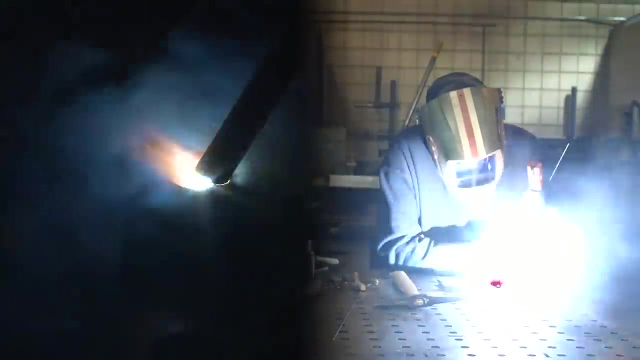 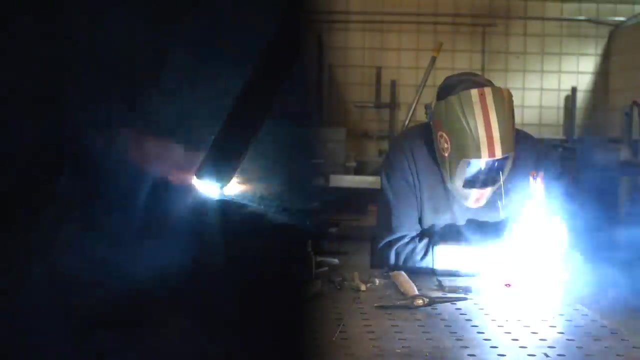 kind of long arc, lift over and bring it back into the top of this pool here and take off again. you know we're back in business again. I think I was just getting ready to say I'm barely dragging the rod, touching the material barely. last thing you want to do. 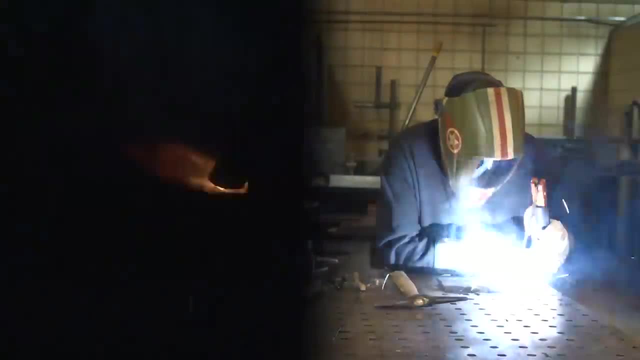 with one of these rods is gouge the plate. now here's something to pay attention to when we come out here and terminate the weld. please do not wait until we come out here and terminate the weld. please do not wait until we come out here and terminate the weld. please do not. 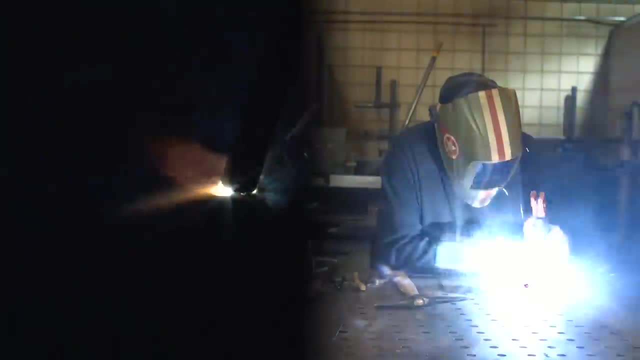 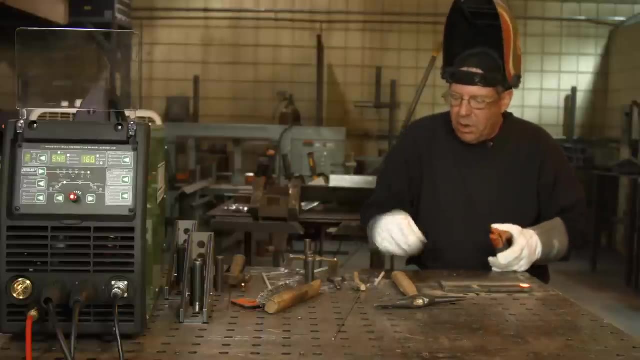 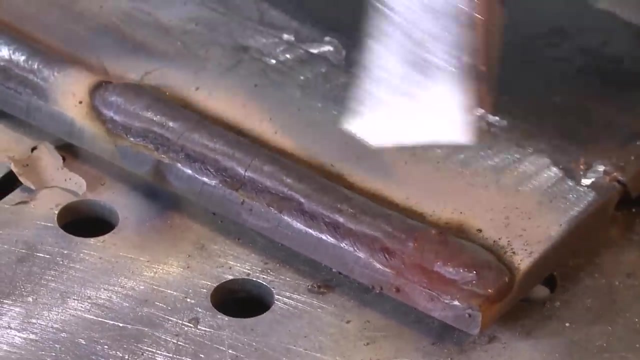 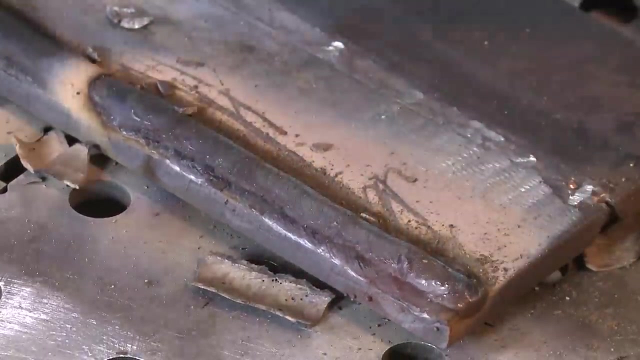 get into the habit of running this crater out here on the edge of the weld and blowing it up. run the rod back in and fill that up a little bit, please, please, do that for me. it's good craftsmanship not getting a slag peel, but it doesn't take much to get this off here. okay, also what this is. 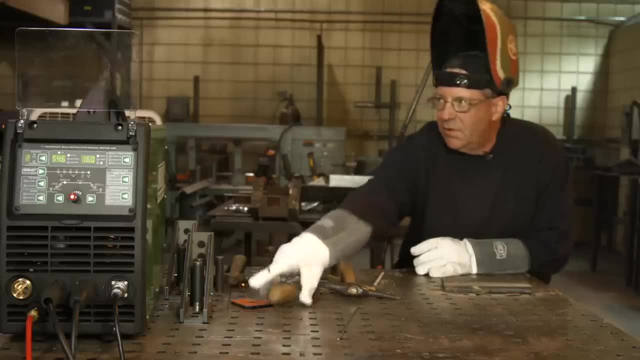 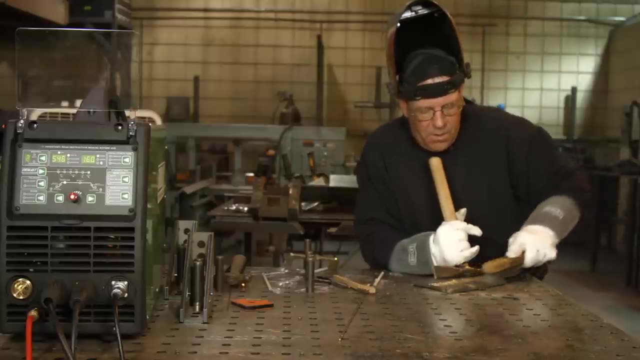 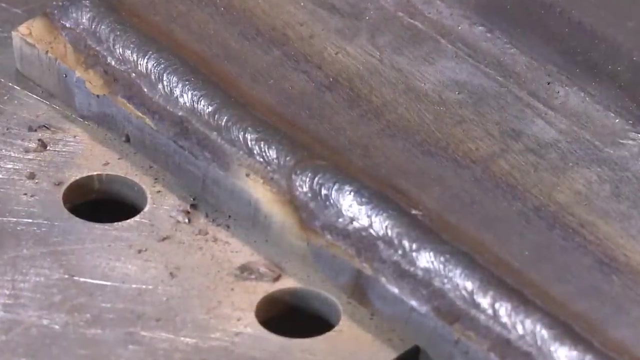 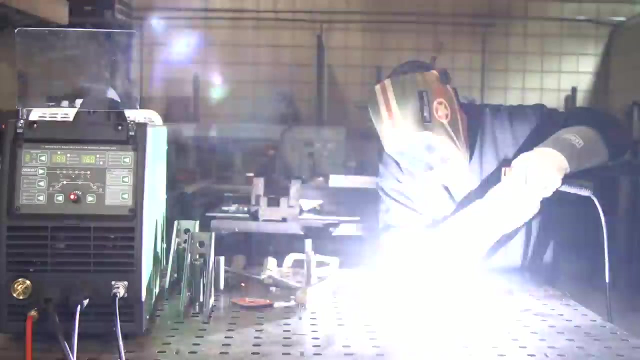 training. you may not realize it yet, but this is training you to run multiple beads when you go to build up. build up a big fillet weld. by the way, right here is our restart, where we stuck the rod. I'm good at sticking rods. I'm gonna run one more. 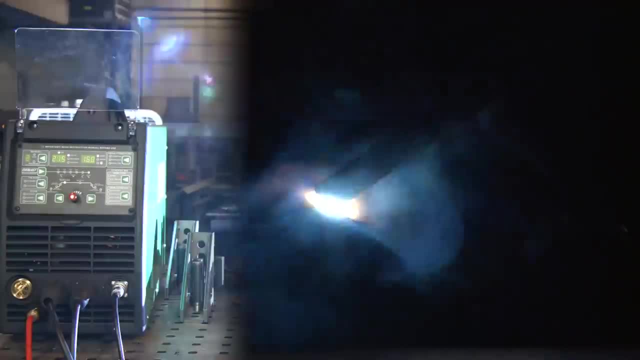 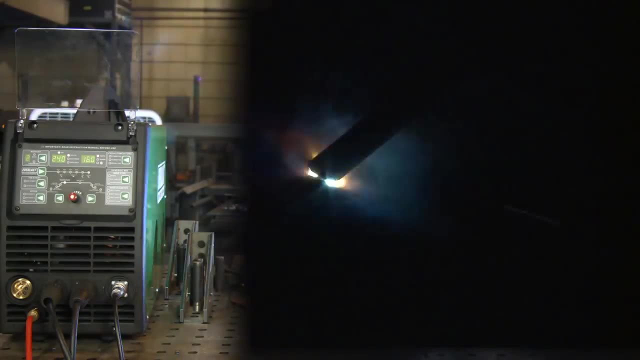 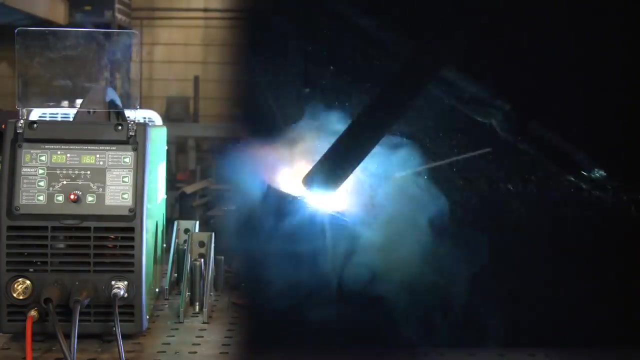 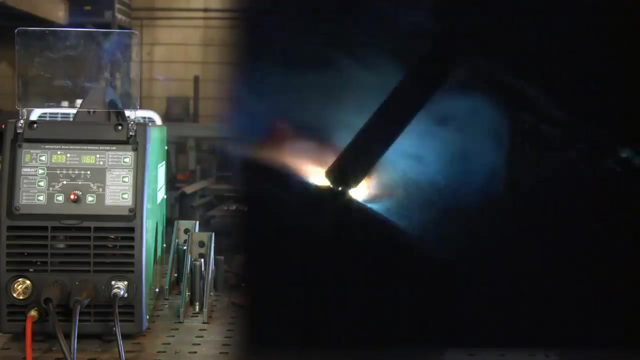 I said I was gonna run one more bead and I'm gonna run two, and the reason is this plate is now getting saturated with heat, so I'm seeing a slight difference in the size of my weld tool. I'm watching the drag lines or the freeze lines. it's where the weld tool turns from bright red dark red. 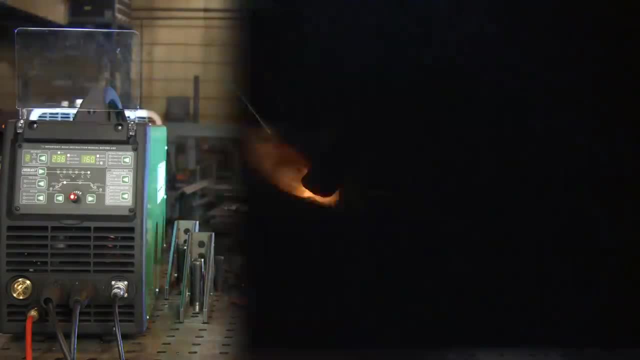 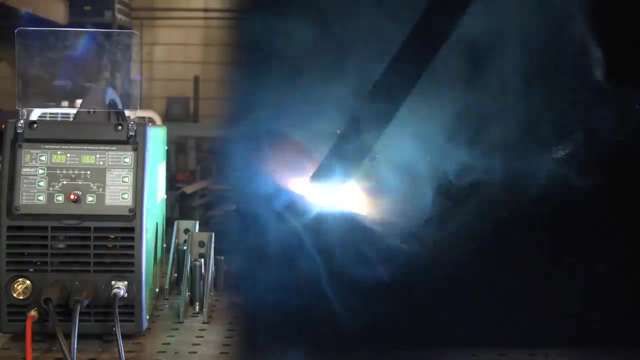 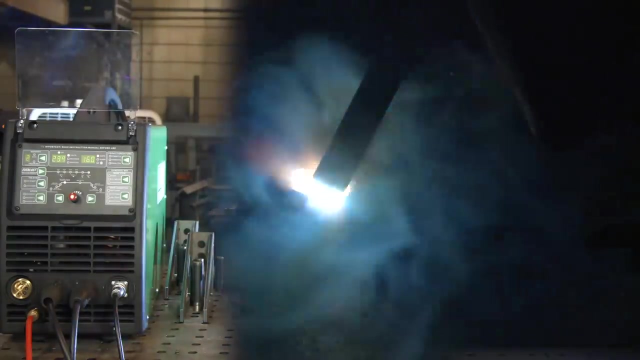 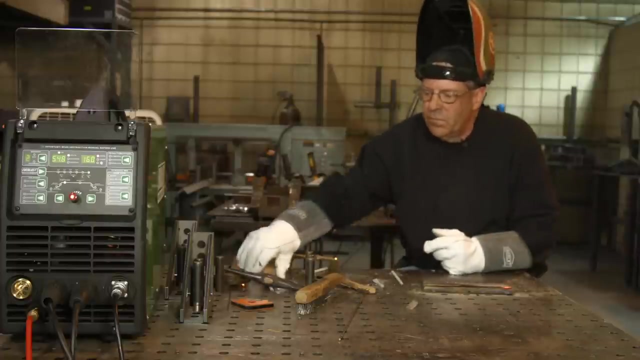 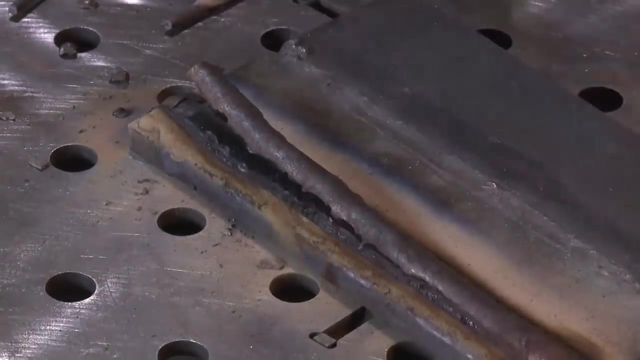 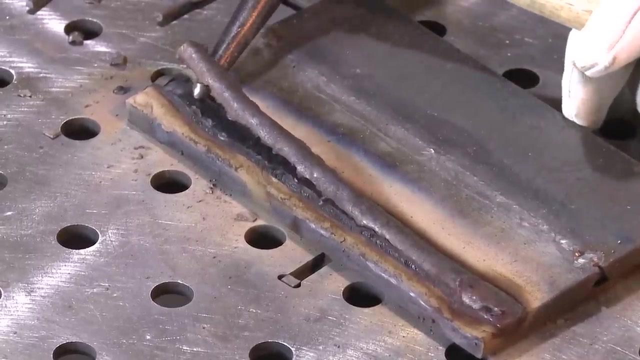 and it's where the weld tool turns from bright red, dark red. hey, looky there, little slag peel. I wonder what this stuff tastes like. Better not. Okay, here's a little slag peel right here. Lookie there, That's always fun. 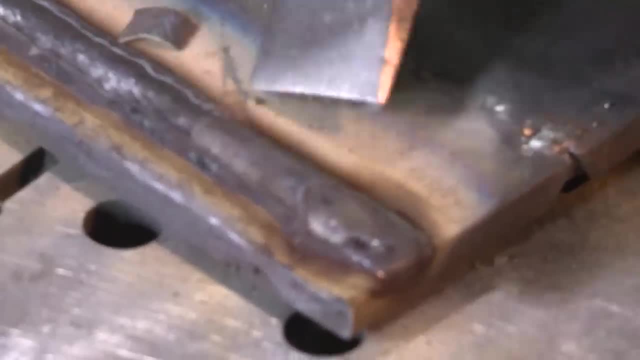 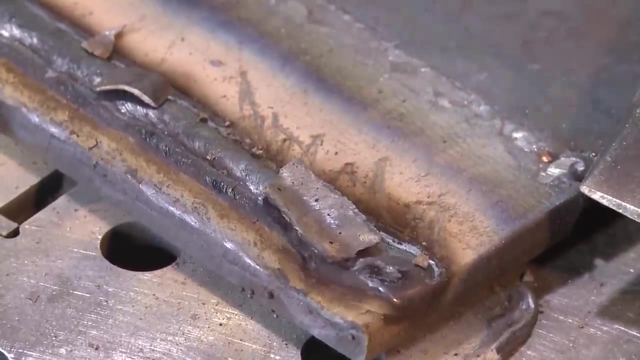 I always like to remove my slag like that. Don't be one to beat the daylights out of your slag If your slag is not coming off your beads, especially these rods right here: 60,, 13,, 70,, 14,, 70,, 18,, 70,, 24,. 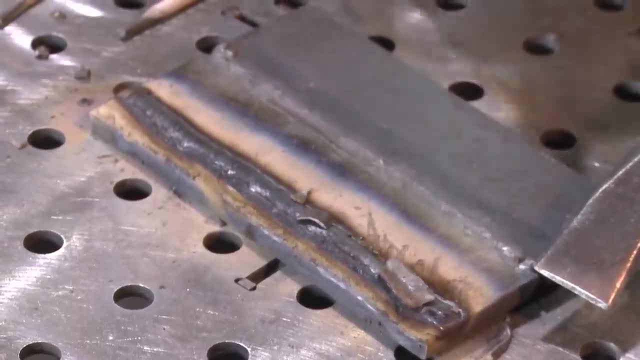 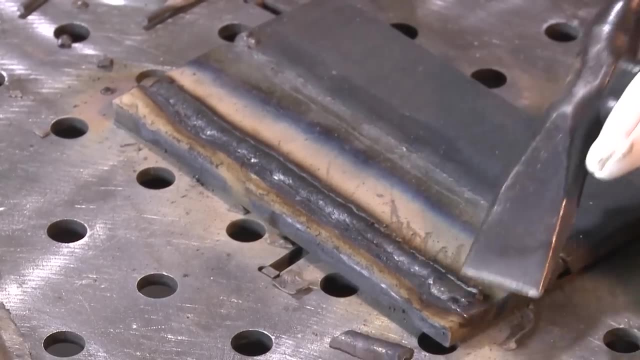 there's no reason to beat the daylights out of it. As a matter of fact, it's dangerous. This stuff stays hot for a long time And I have actually been wearing safety glasses, face shield, and I've got stuff in my eye. 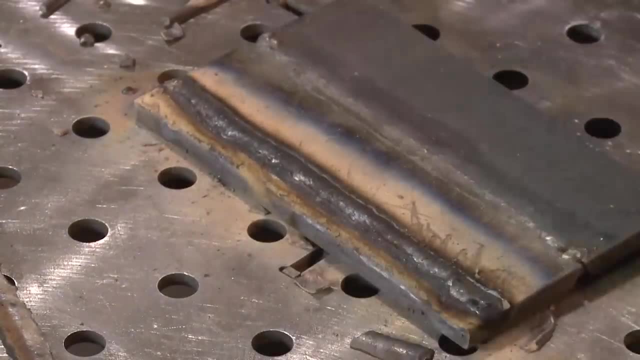 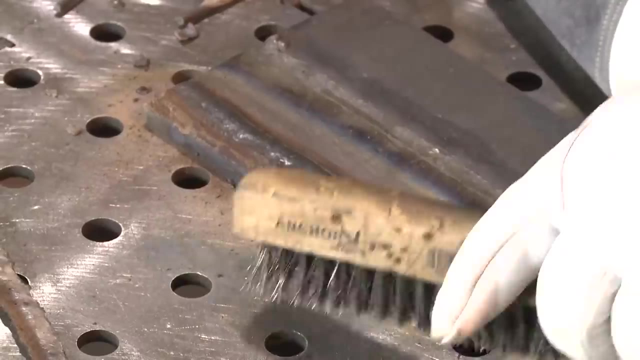 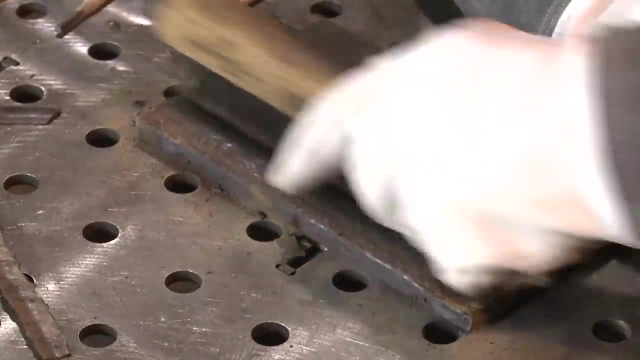 So just kind of avoid the projectile part of welding and don't beat on stuff. Plus, it makes it a lot quieter in the weld shop and your welding instructor will appreciate it. Nothing makes a welding instructor more irritable than somebody banging around on the plate all the time. 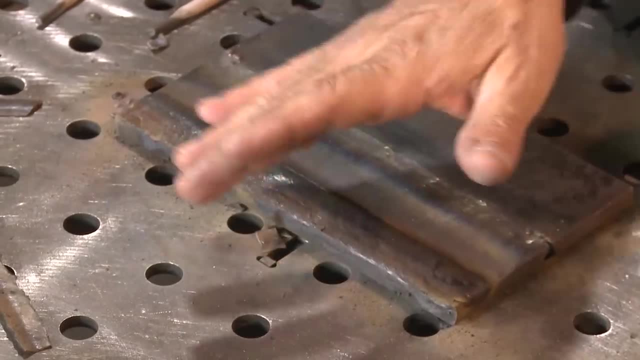 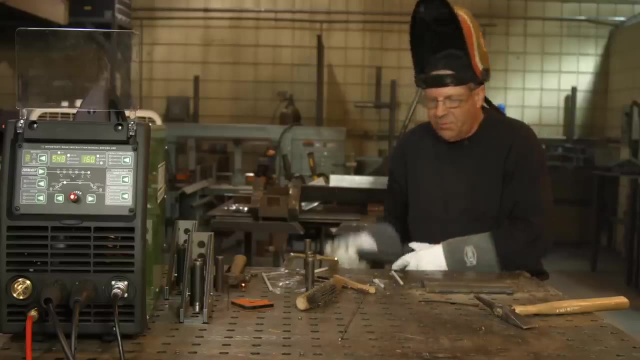 Okay, I know this rascal is super hot, super hot. I'm gonna leave the machine the way it is- 160 amps- but I'm gonna go take all the heat out of this plate. okay, I'm just gonna dip it real quick. 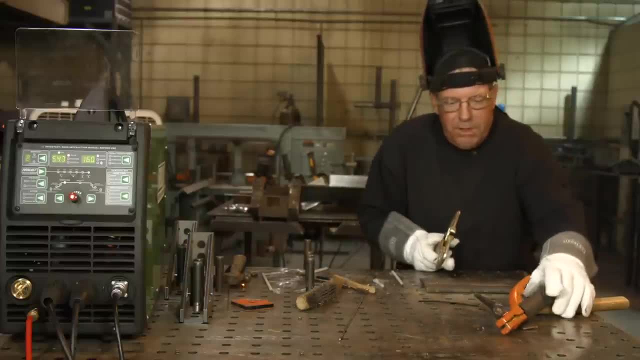 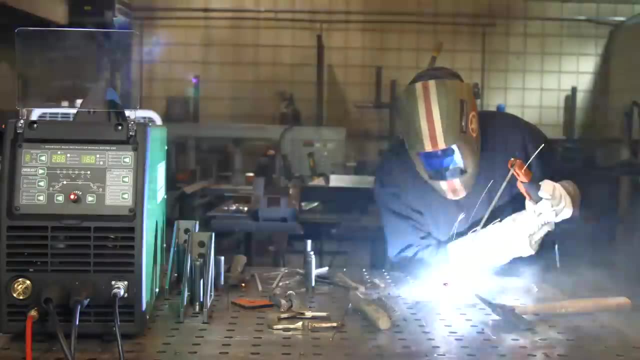 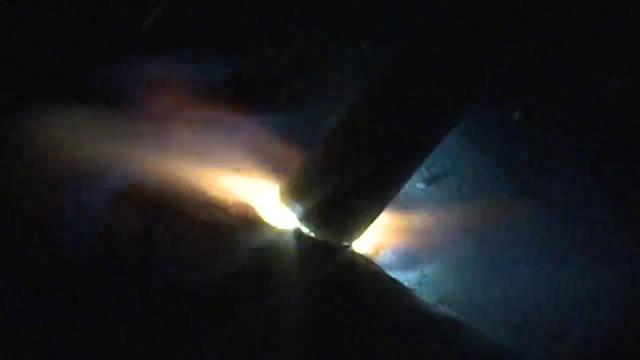 I just wanna get a lot of that latent heat out of there. Be right back, Come on. I must have a slag coat on the end of these old rods here. Okay, I went over and cooled the plate off. I left the amperage alone. 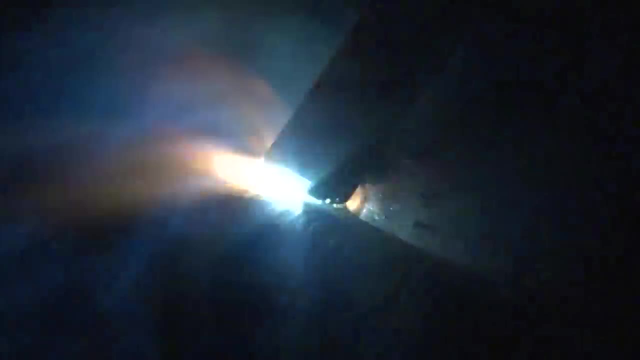 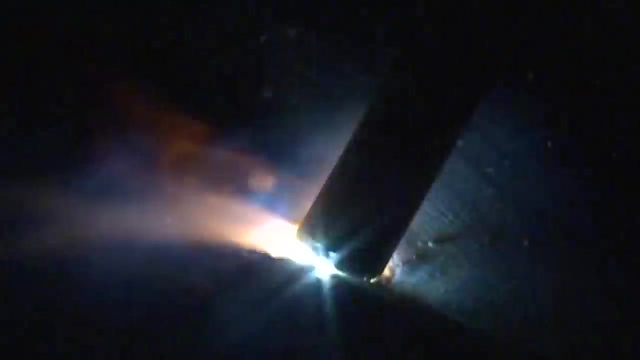 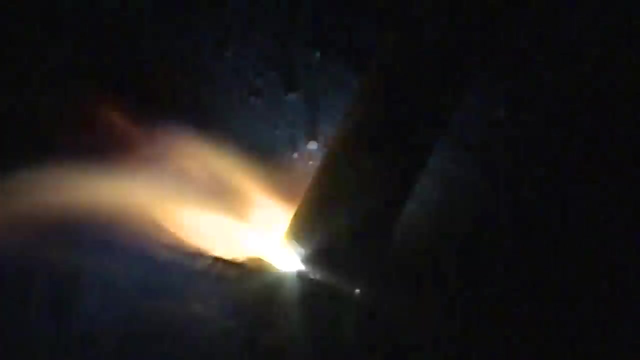 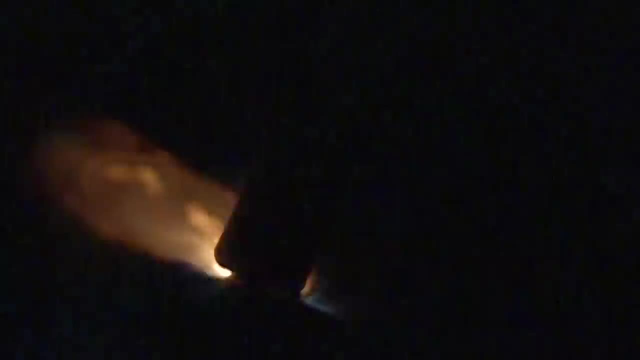 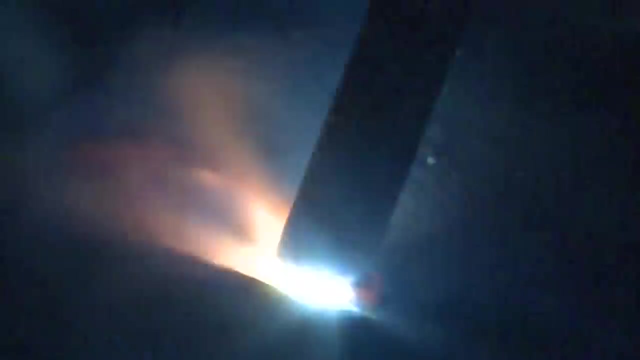 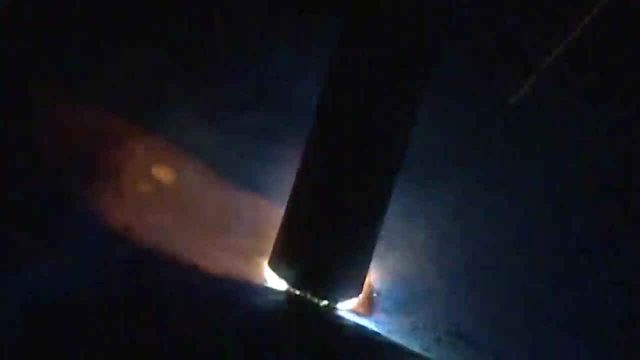 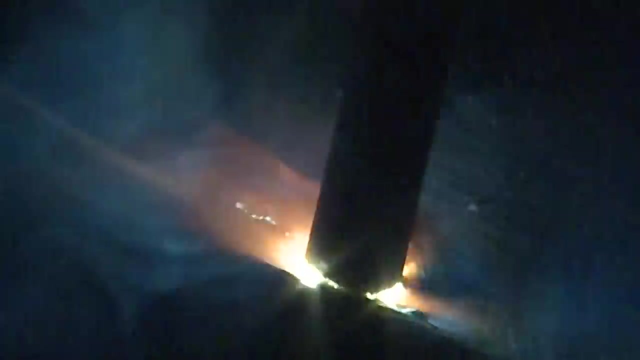 I'm using it as a guide. If you see me weaving slightly back and forth because I'm old and not quite as steady as I used to be, Oh yeah, that's my excuse anyway. Wow, it's almost like I'm not gonna make it all the way. 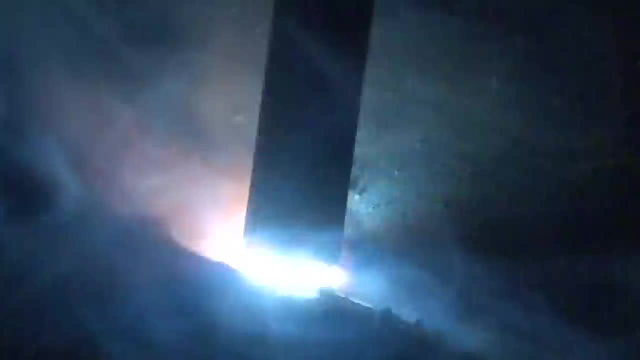 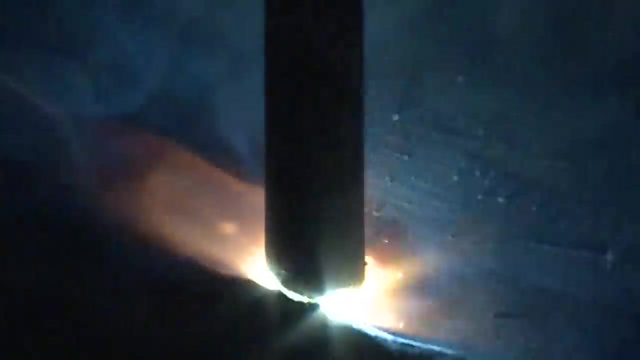 Oh, that was a nice little explosion. Just like this rod isn't gonna make it all the way to the end, Maybe it will Gonna be pushing it. One thing about it is I'm not gonna speed up If I run out of rod. I run out of rod. 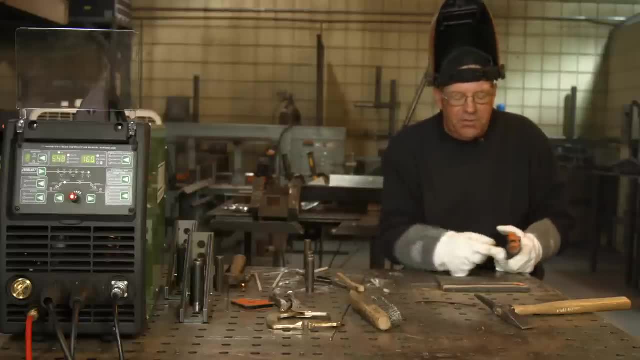 Barely made it. That's another thing I see people do. They can see where the end of the plate is and they know they're running out of rod, so they hurry up and get over there and it changes the width. It changes the width of their bead. 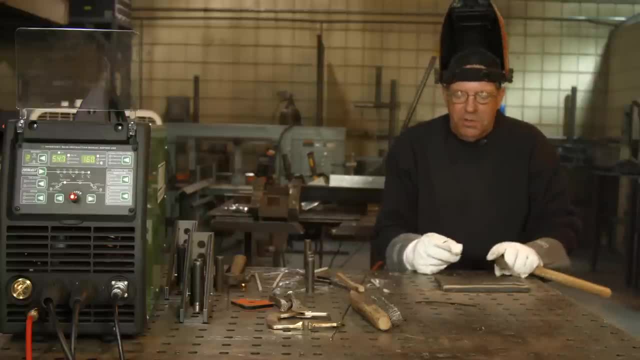 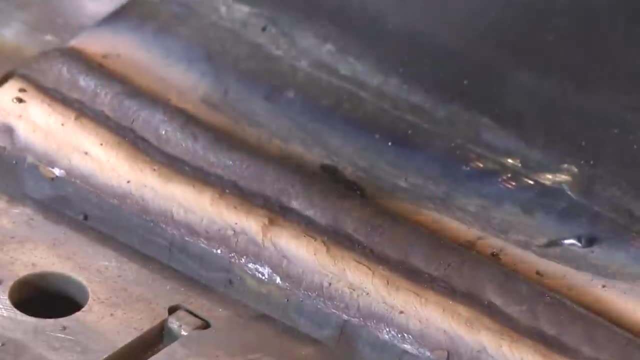 Don't do it, Don't do it. You need to practice restarting anyway. When that electrode exploded a minute ago, it left a nice little oh, but it's loose. Okay, I'm good. See, I'm not getting a slag peel this time. 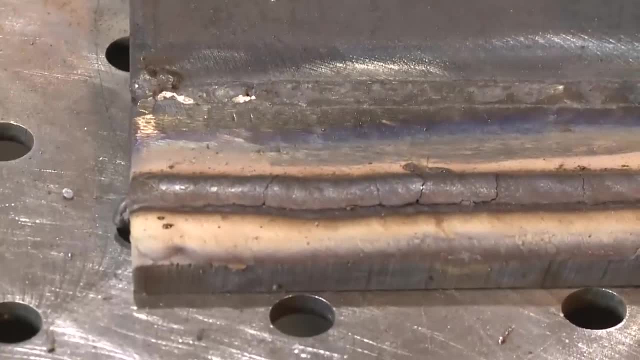 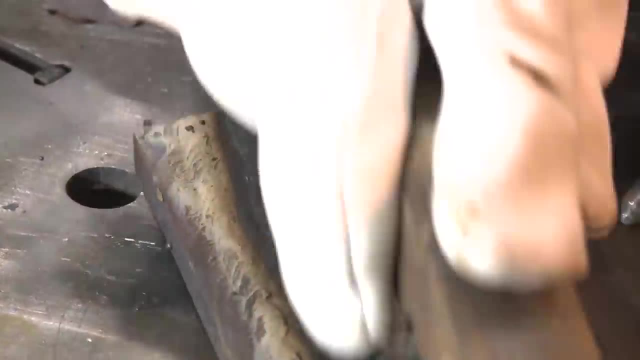 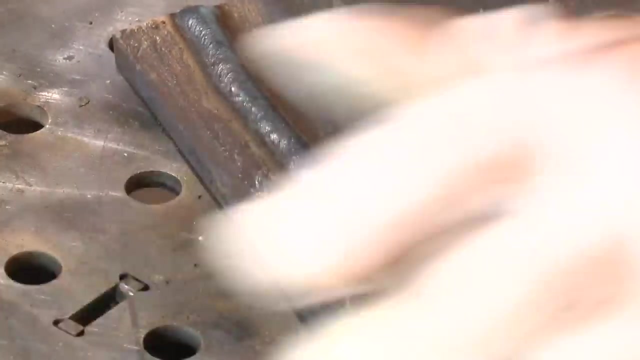 but my slag is cracked and it flew right up off there for me. Okay, I'm gonna brush the toe of the weld. I'm gonna brush the toe of the weld. I'm gonna brush the toe of the weld By doing this method. I know this seems boring. 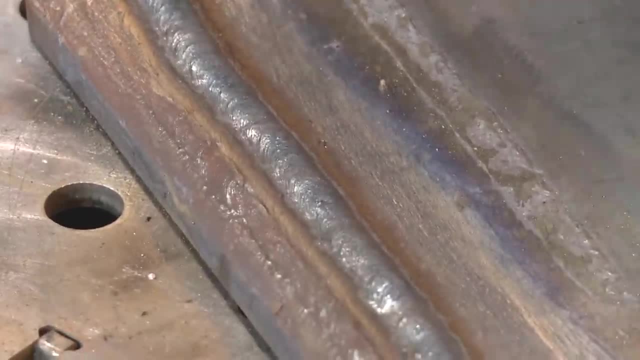 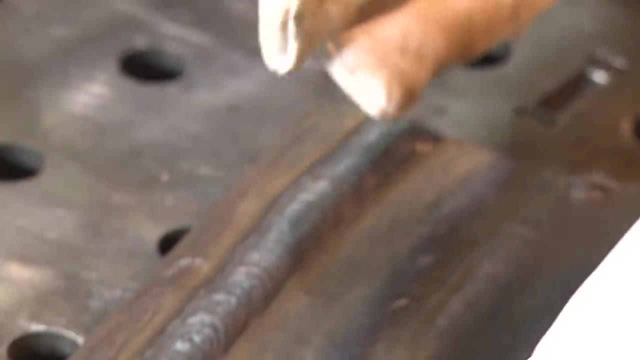 but you need to challenge yourself. Run the exact same straight line. Run as straight as you can possibly run. I'm starting out and I've already got a little curvature to mine. I could correct it by I could- eh, I could do it. 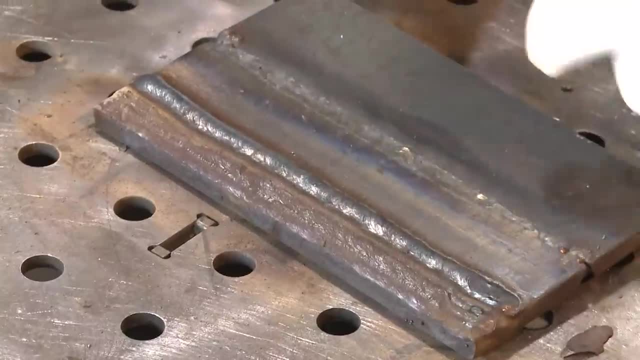 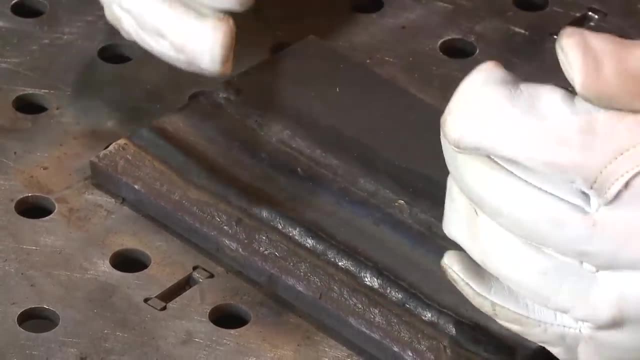 You know it's okay to run a straight line. Grab a piece of soapstone and leave yourself a guide mark in there. Whether you do it, whether you measure it off of here, just make a straight line so that when you run in the toe of the weld, 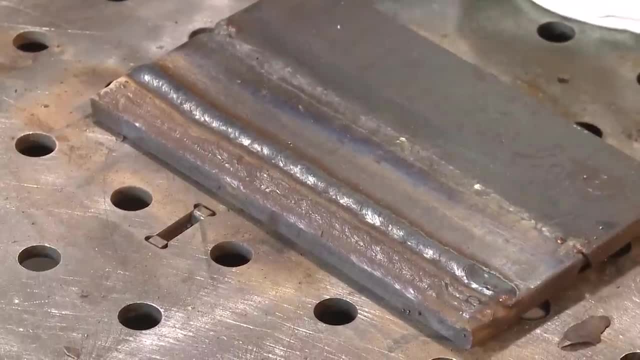 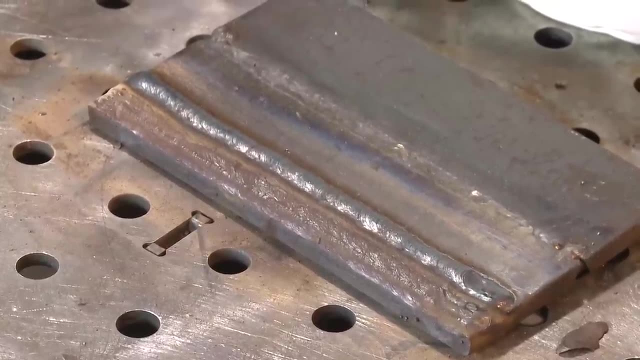 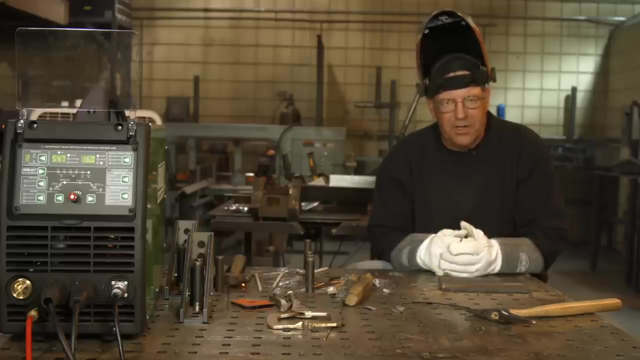 you can kind of pause or do something and then you'll straighten them right back up. But challenge yourself to run really straight beads, because when you get into stacking multiple passes they need to be the same size, same width Here I'll just throw this out there: